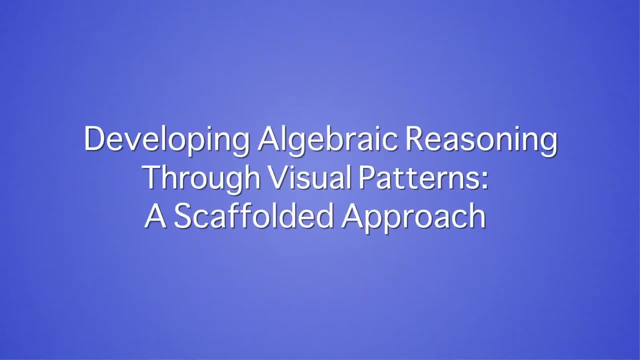 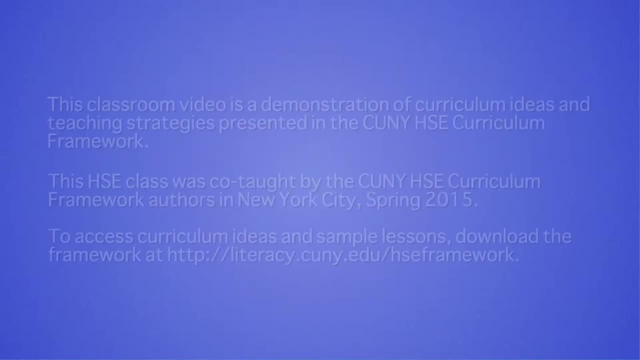 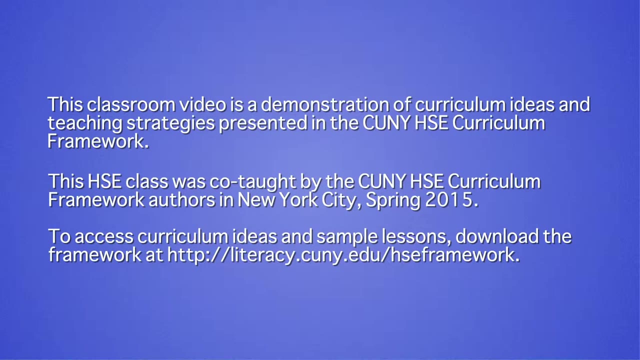 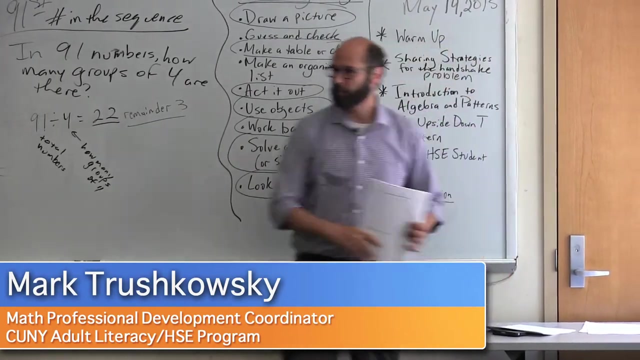 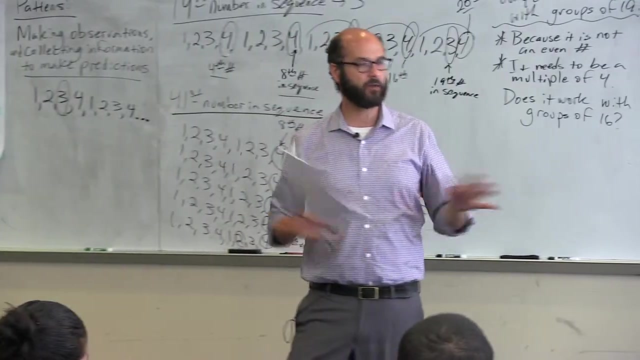 So we're going to look at something that's not a number pattern, but it's a visual pattern, It's a picture that's changing. Just take a look at the first two questions, okay, And then you guys are going to come together, But on your own, just give yourselves a little bit of time to really look. 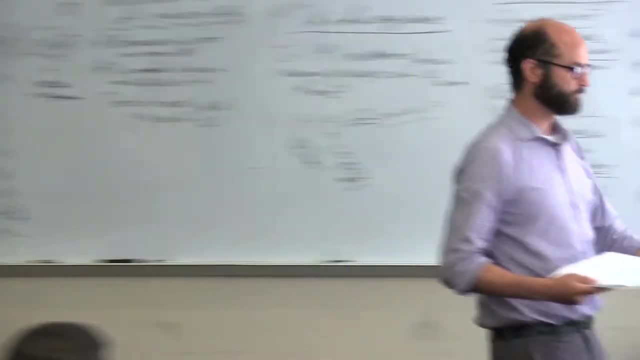 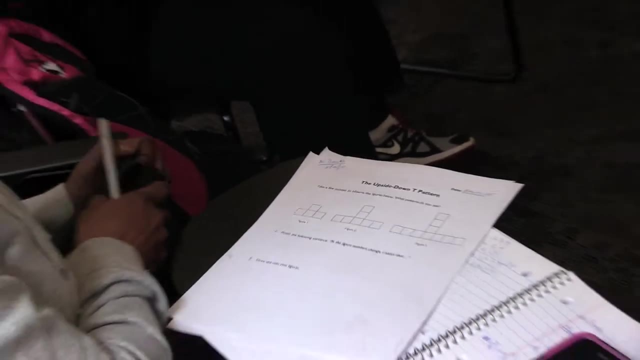 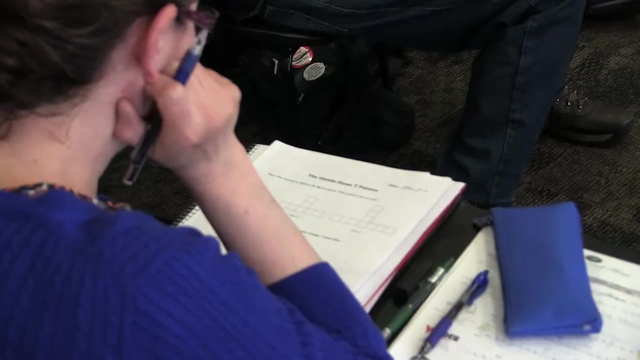 at what this is okay. What patterns you see? here Today we looked at a t-shaped problem. It's really just about pushing them to see as many different patterns as they can, because the more patterns you identify, the better your prediction is going to be. The series of questions that they answered. 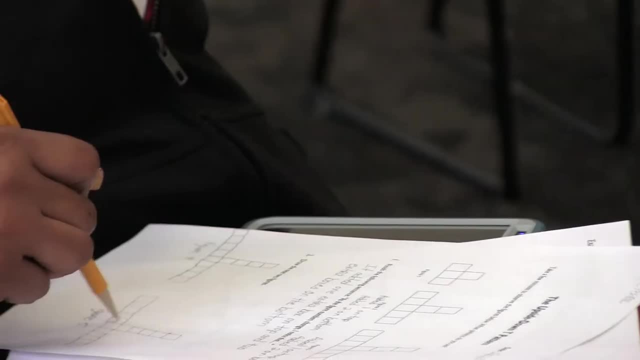 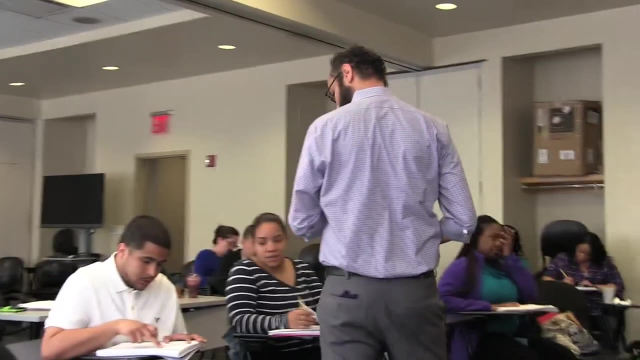 today, which is: what patterns do you see? What are the next two figures look like? How would you describe what the 10th figure would look like? And then the 46th figure? what's that going to look like? The final question is going to be: how would you figure out the number of squares in any 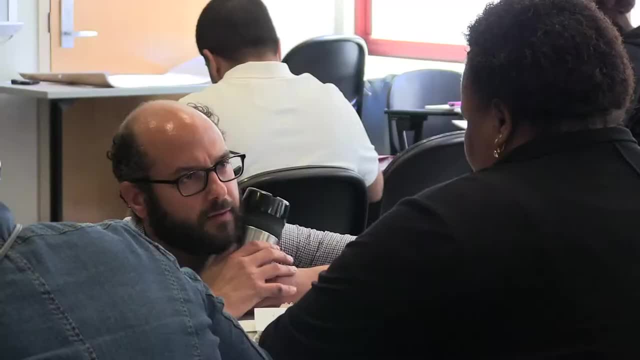 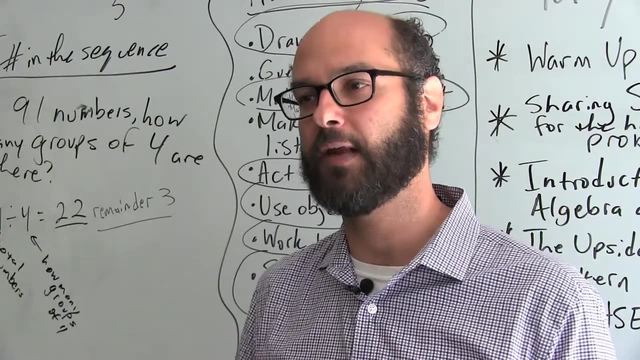 pattern right And to start moving into variables, so that the idea is that that algebra is a tool and algebraic thinking is a way of thinking. That's our way in. So that's why we're focusing on patterns: to develop it as a way of thinking, not just a discrete set of tools. You're going. 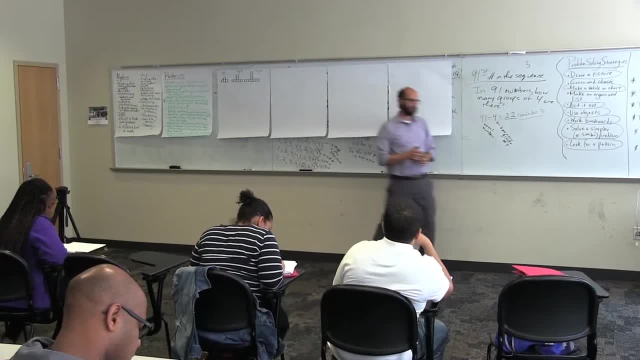 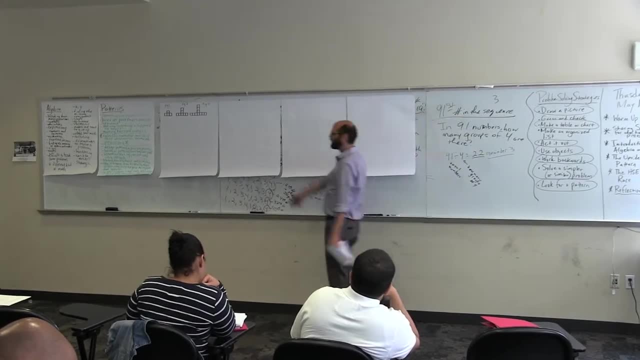 to see how it all fits together. So what patterns do you see On the front here? How did you finish that sentence? As the figure numbers change. so, as it goes from figure one to figure two, to figure three, as the figure numbers change. 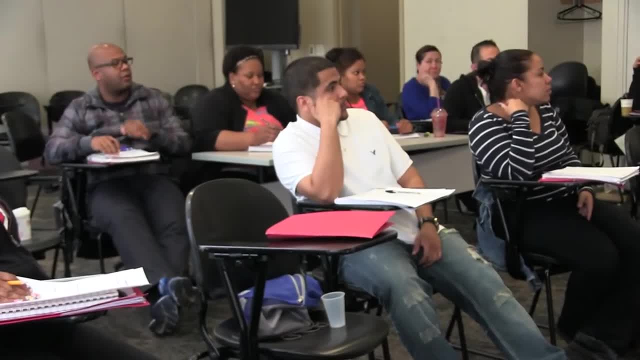 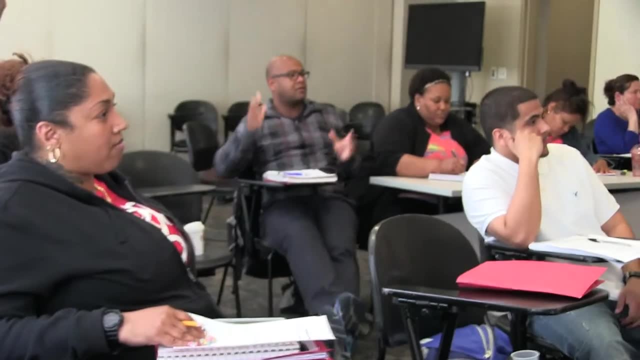 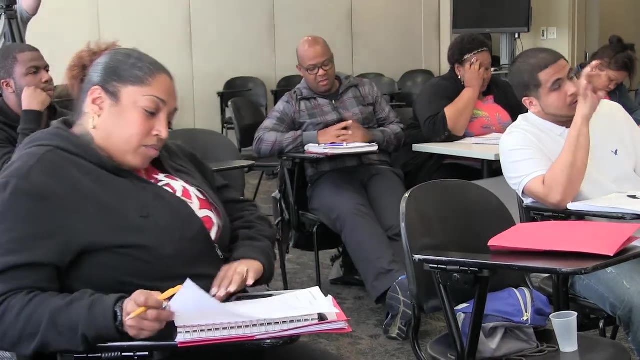 I notice that. what? What did you guys notice? Give me a second, Increased by three. Fabio said it increased by three. What increased by three? The figures increased by three blocks each. We started at four, then it goes to here seven, then it goes to ten and then it goes. 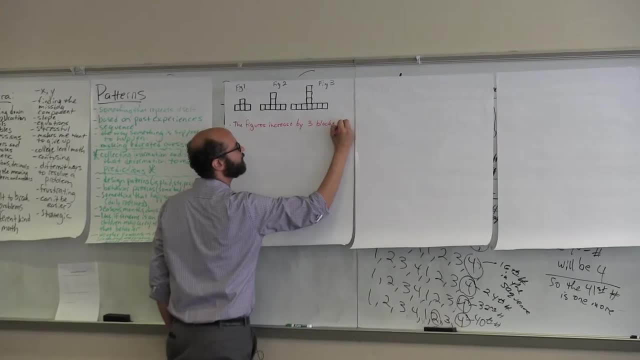 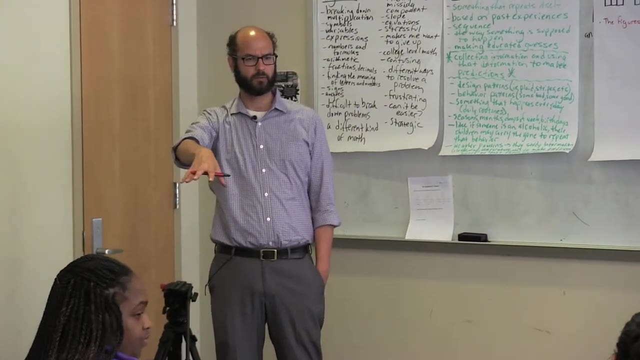 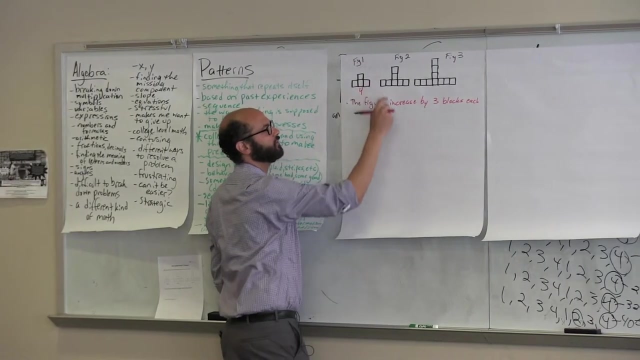 The figures increase by three blocks each. Does everyone agree with that? There's lots of different ways. So he said the first figure has how many? Four, Four. So this one has one, two, three, four, five, six, seven. 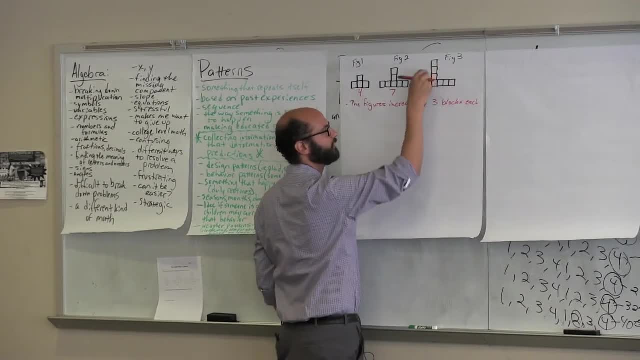 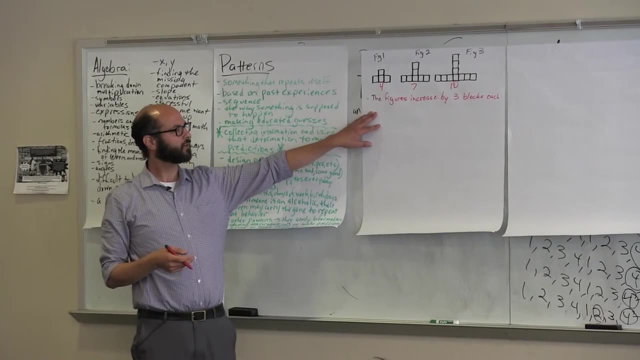 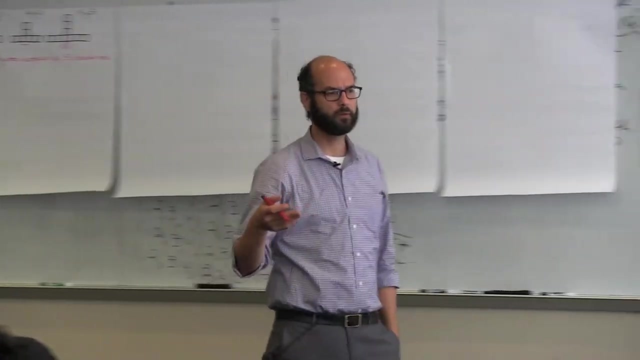 So this one has one, two, three, four, five, six, seven, eight, nine, ten Right. So why is that a pattern? The figure is increased by three blocks each. What do patterns help us do? Four plus three each time. 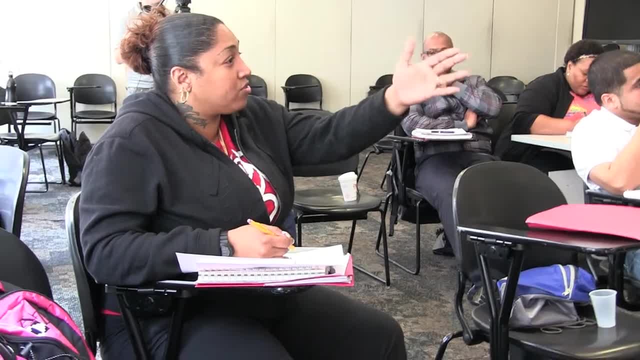 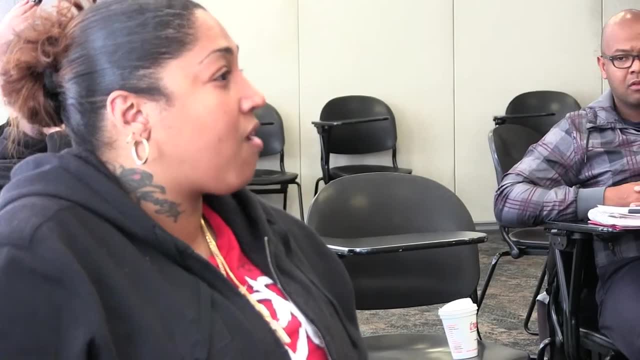 It's four plus three, I mean three Like. four plus three equals seven. Seven plus three equals ten. Right, And what Seven plus three? And then what Thirteen. So the next figure is going to have thirteen right. 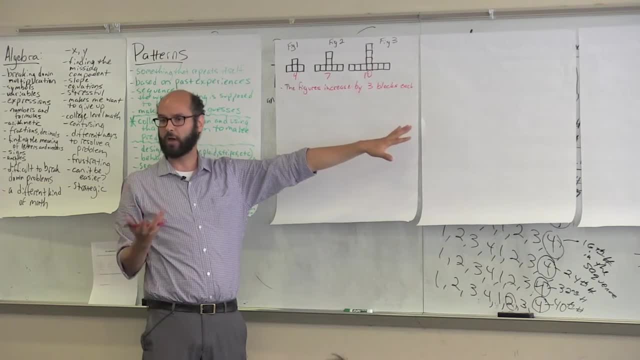 Now do we see the next figure. So how do we know? We're going to create it, We're going to draw it, We're going to draw it, We're going to draw it out. But how do we know? How do we know our picture is correct? 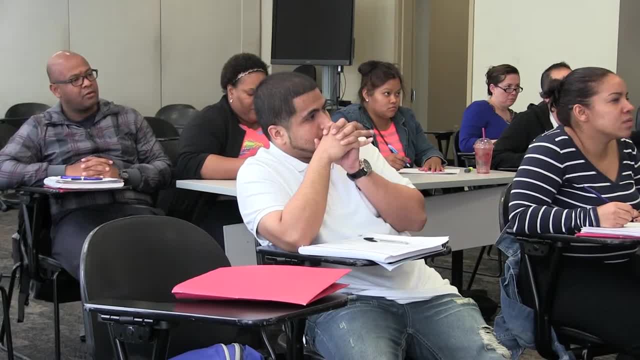 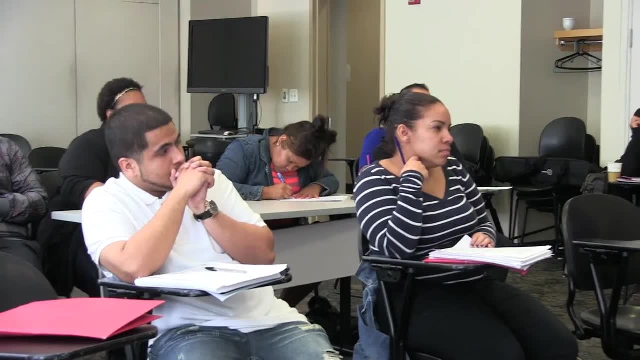 How do we know it's going to have thirteen? Because you add three more, Right? Because we have this pattern. The pattern that he's seeing is that we're going to add three more, so we can use it to make a prediction. Add more boxes to the top. 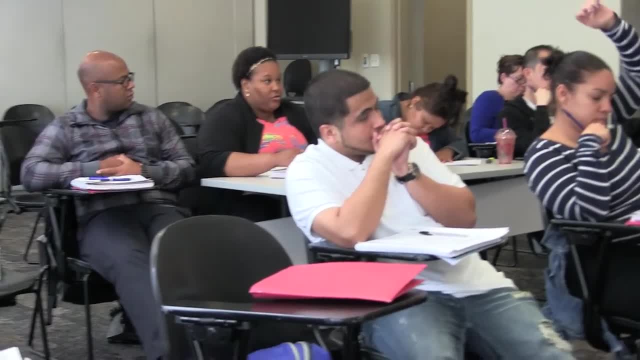 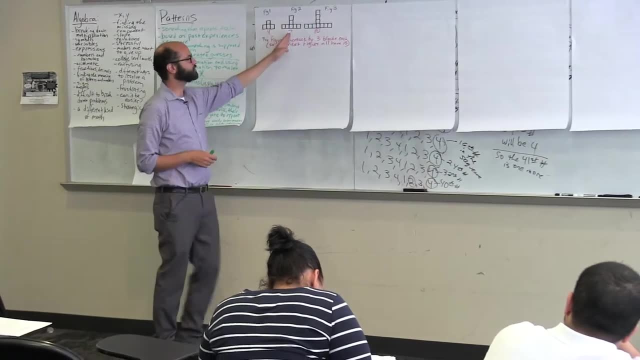 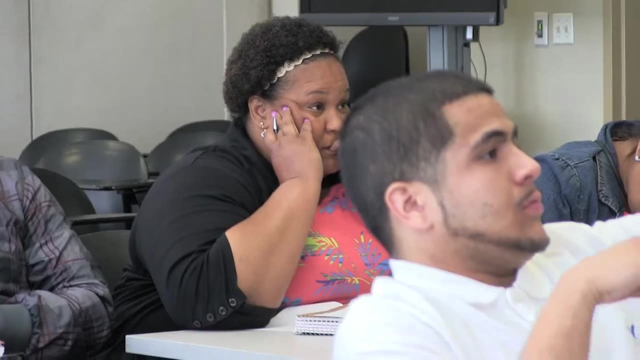 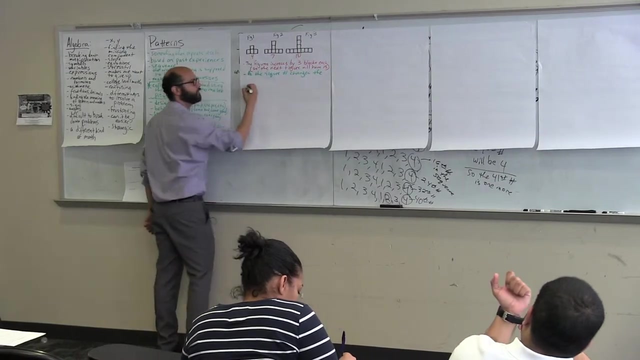 What's that mean? So you make your, do your drawing and add a top. Maybe start with that sentence starter. So, as the figure numbers change, what do you notice changing about the top? It's getting higher. Okay, So as the figure number changes, finish that thought. 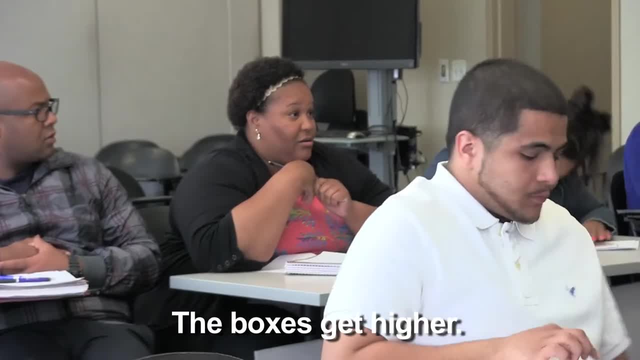 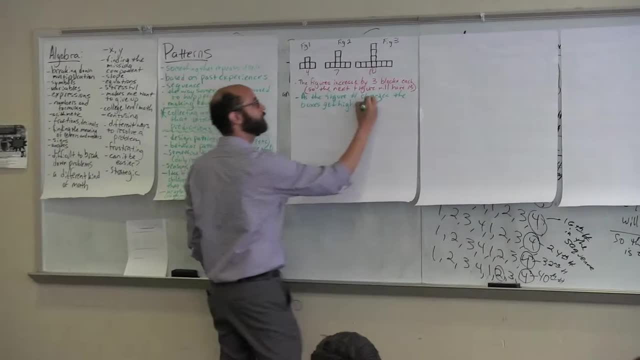 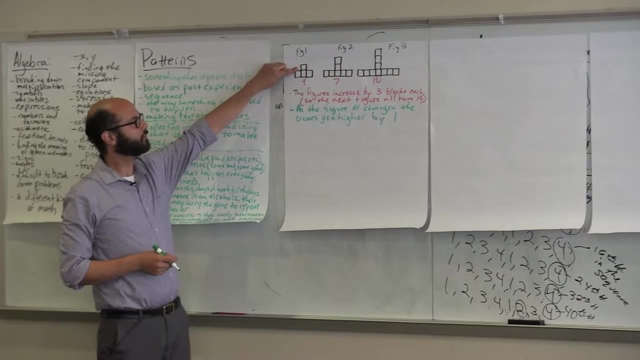 As the figure number changes, the box gets higher. And can I do LaShonna? can I add her? Rene's by one? Yes, Can you say that one too. So how many are in the here? One One. 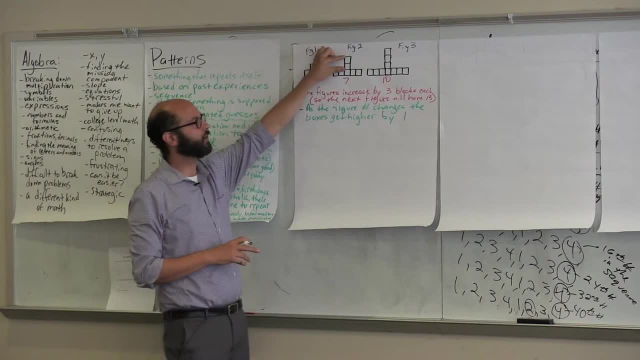 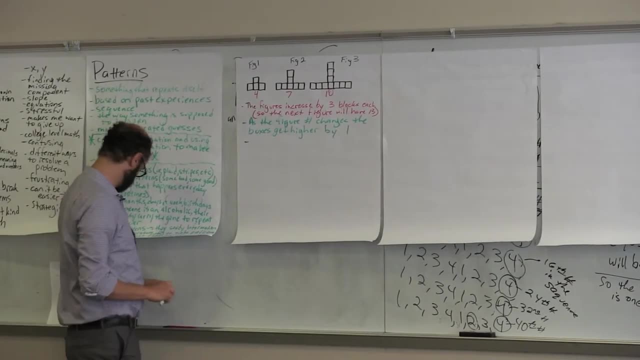 Or two, Depending on how you look at it. So there's one on top. How many here? Two, Two here. So the next figure would have Four. Would have four on top. Okay, Another way I put, more boxes were added and the T got bigger. 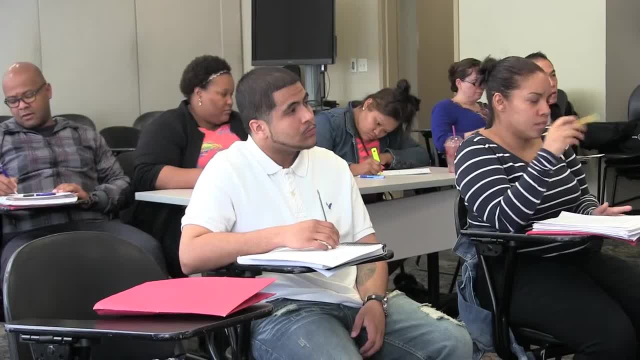 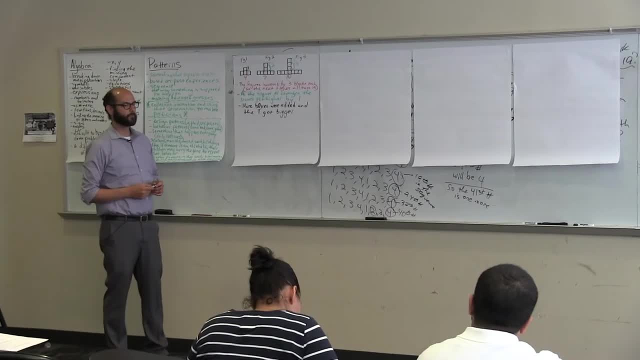 Okay, So more boxes were added and the T got bigger. Good, What else? Yeah, Roxanne, All the boxes have equal amount of boxes, except for that middle one, If you don't count the one that attacks The T, they all have the equal, same amount of boxes. 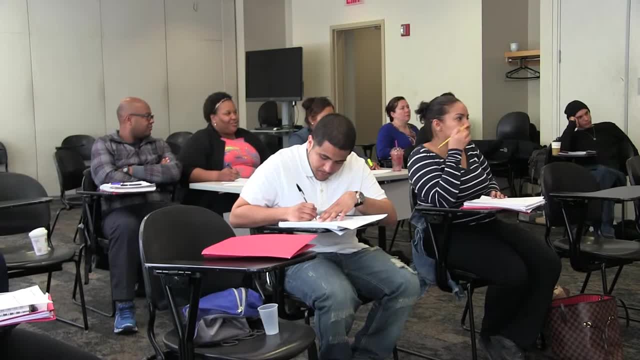 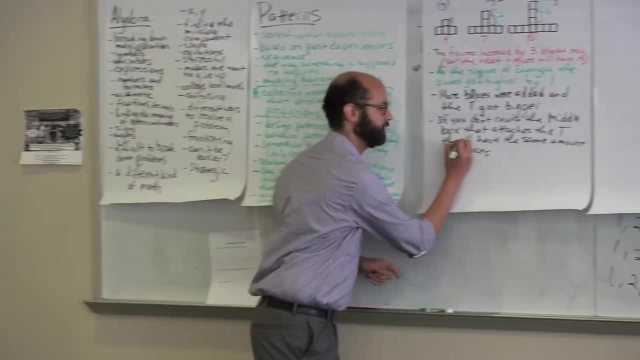 What do people think of that? Is that true for each one of these pictures? If you don't count On either side, If you don't count the middle box that attaches the T, sorry, They all have the same amount of boxes. 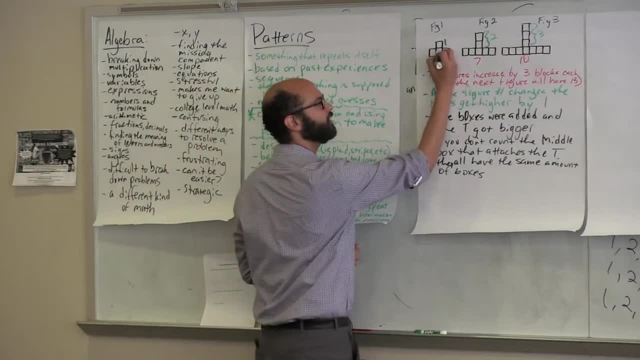 So let's, let's. maybe you mean this is the box That you don't count. So if I don't count that On the side, And if I don't count that They have the same amount, And if I don't count that, 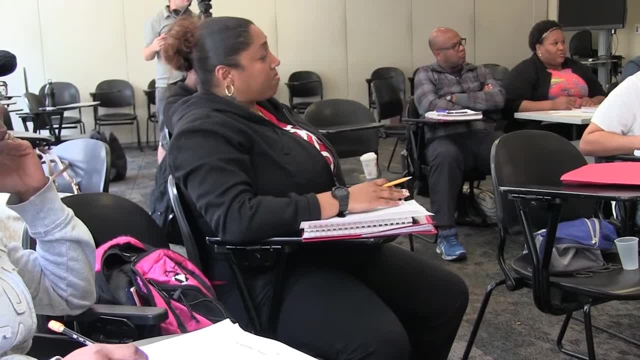 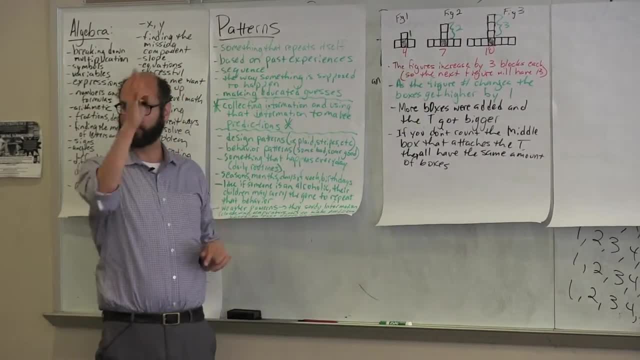 They have the same amount. And if I don't count that, If I don't count that, that's what you're saying, So if I don't count, so, Sandra, if I don't count the box that's colored in, do they all have the same amount of boxes? 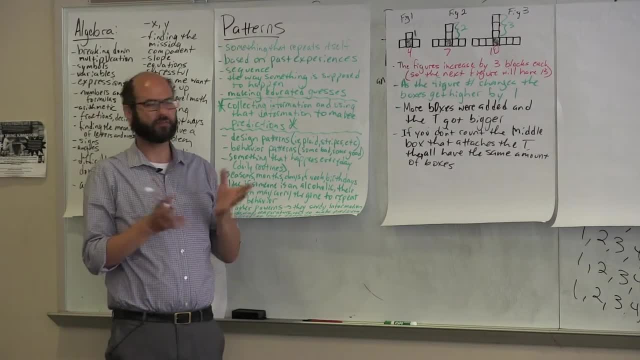 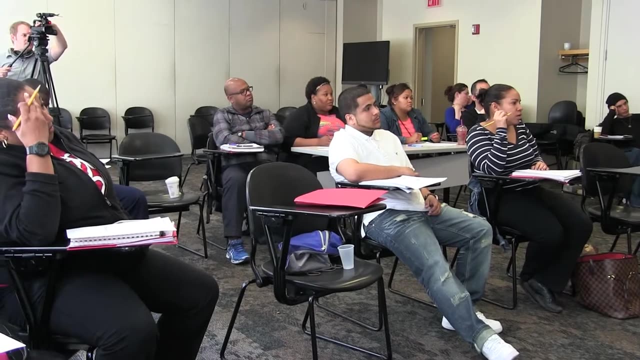 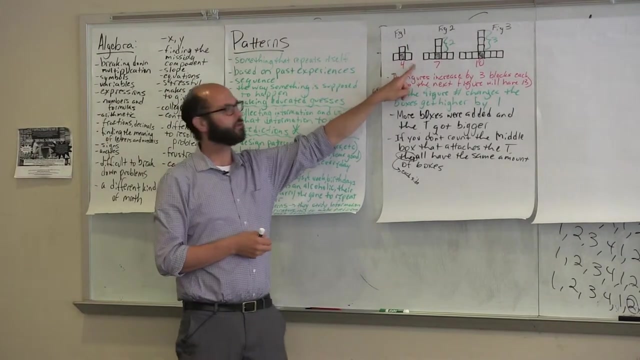 Yes, What? What has the same? when we say Each side, Each side is even. You got one, two, one, two, one two. So they, by they, we mean each, Each side, Each side. So this one is one, this one is one, this one is one. 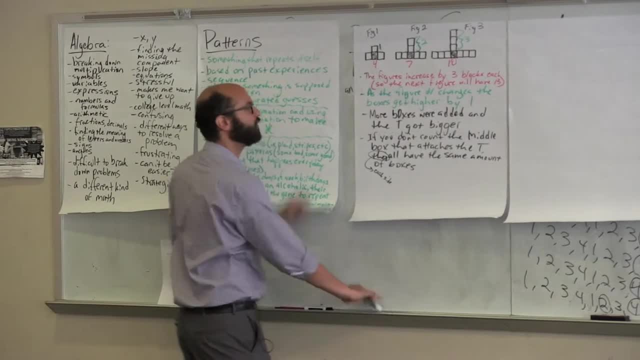 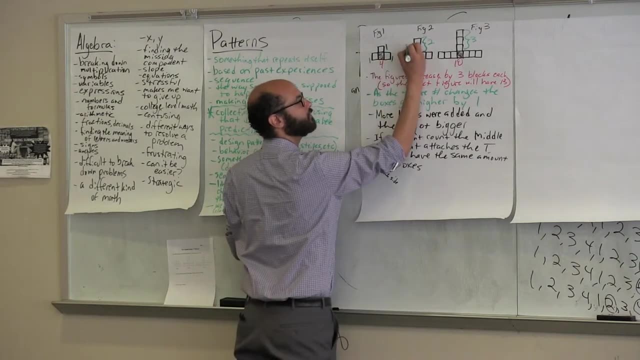 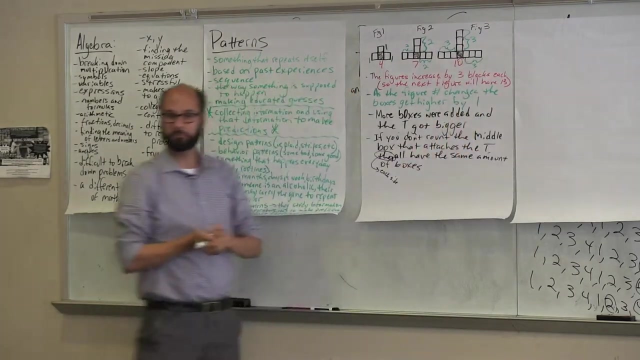 This one is two, this one is two, this one is two. So it's kind of similar to what LaShonna saw going up, but it's also one one, one, two, two, three, three. OK, You keep adding one box to each side. 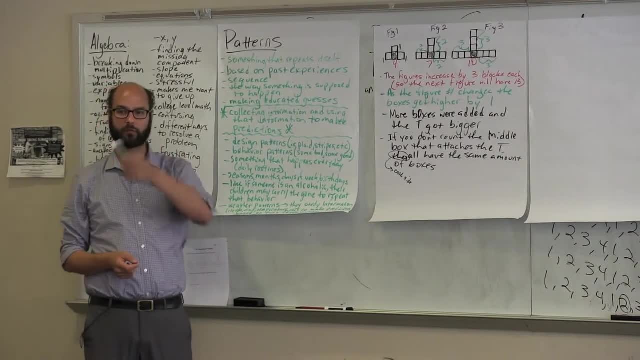 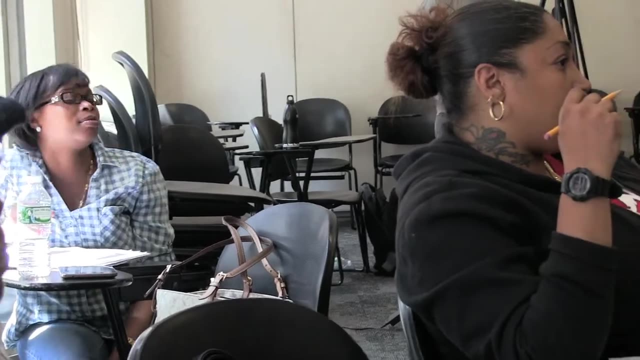 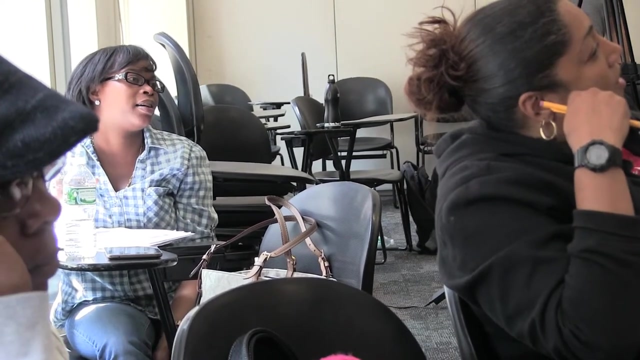 OK, Good, What else At the bottom? the first one is three, So the first one is three boxes. OK, The second one is how many boxes across? One, two, three, four? I think it's five, Five. 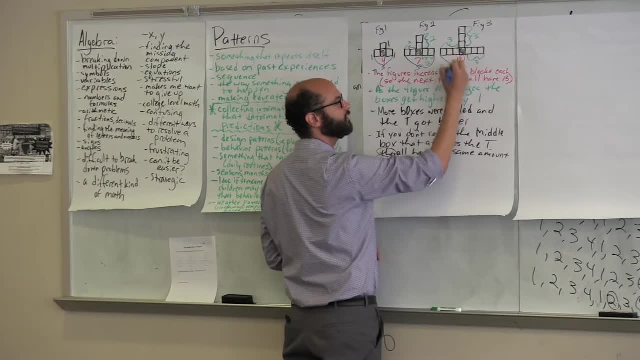 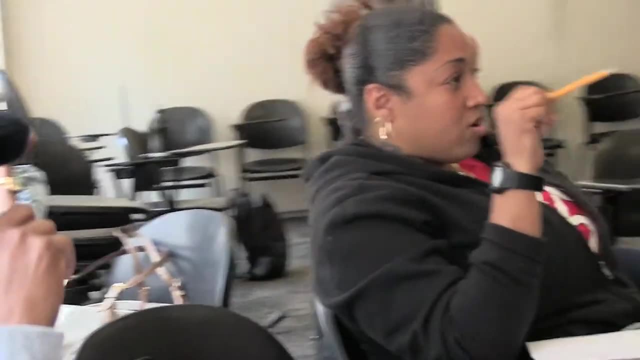 And this next one is one, two, three, four, five, six, seven. So how can we put that in words? And each one is adding one on top and two on the bottom. But let's stick with the bottom first. 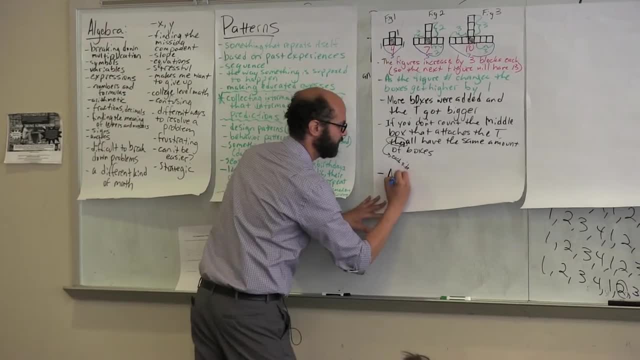 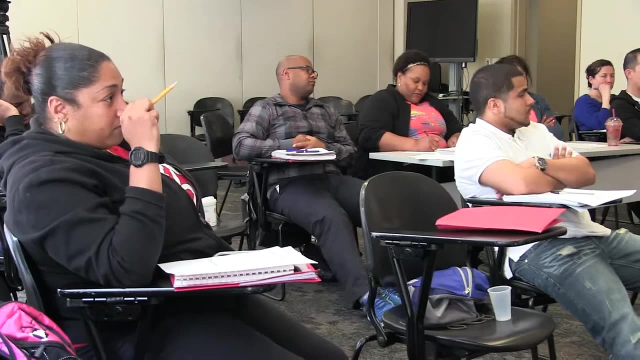 So, as the figure number changes, say that again, Roxanne. OK, OK, The top one is adding one, But let's stick with this. It's adding two on each side. So as the figure number changes, I'm adding one on each side. 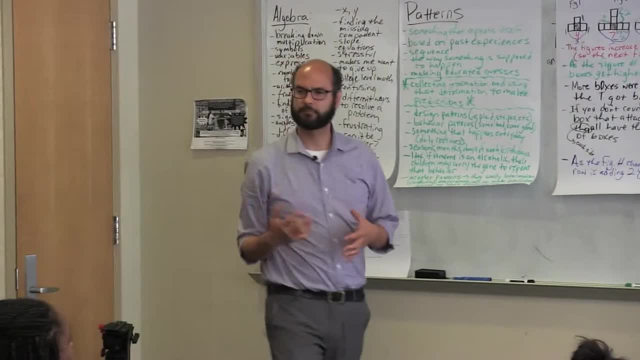 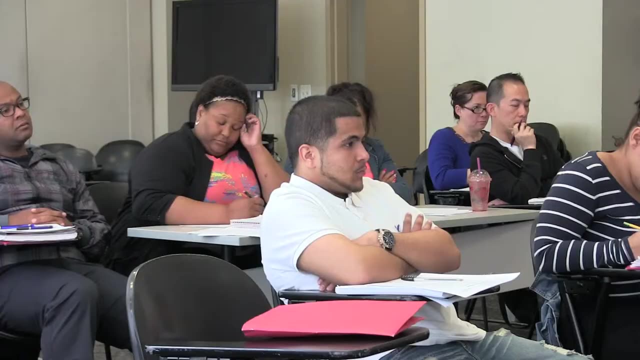 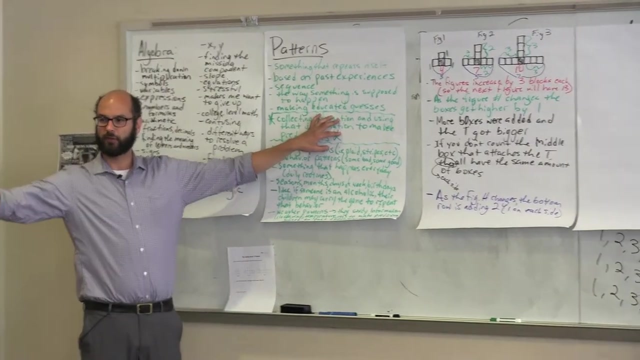 So which one is the right pattern? Which one is the right pattern? They're all right. They all are right. The idea with patterns, we're collecting information and using that information to make predictions. We don't know what information is going to be useful, right. 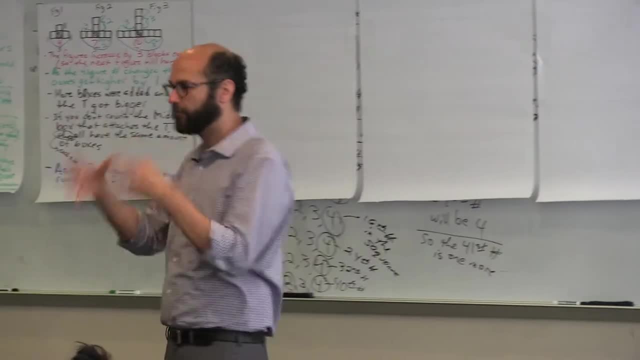 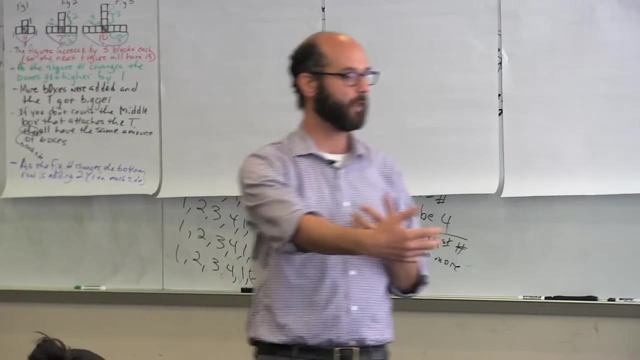 You want to gather, see all the different pattern, as many different patterns as you can, Because the more patterns you see, the more information you're going to have to make a better prediction. OK, So if we, for example, only had one of these, we said: 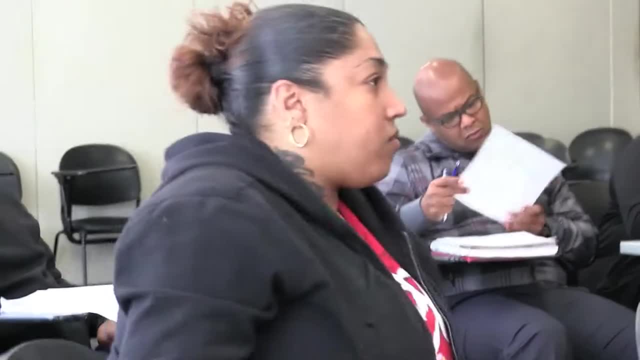 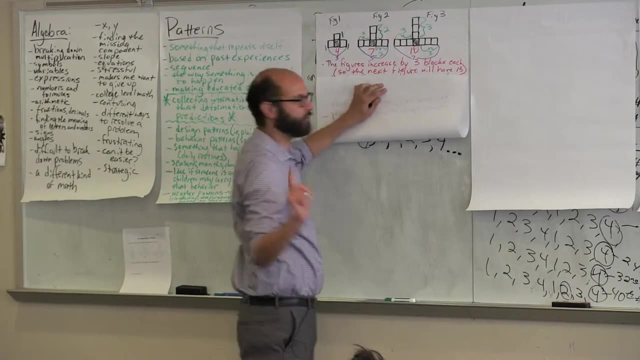 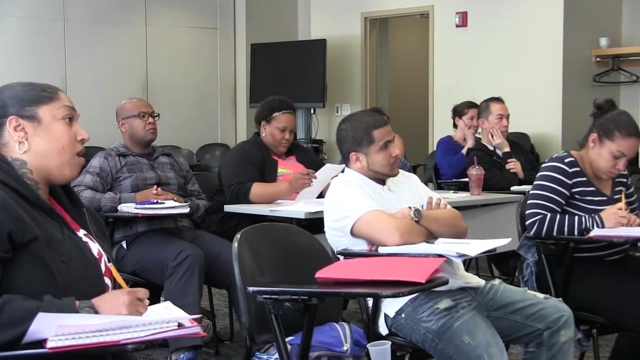 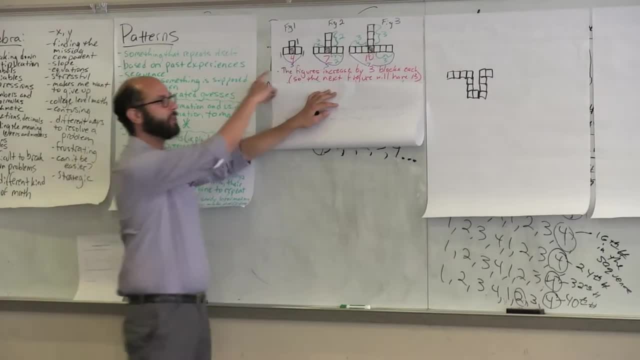 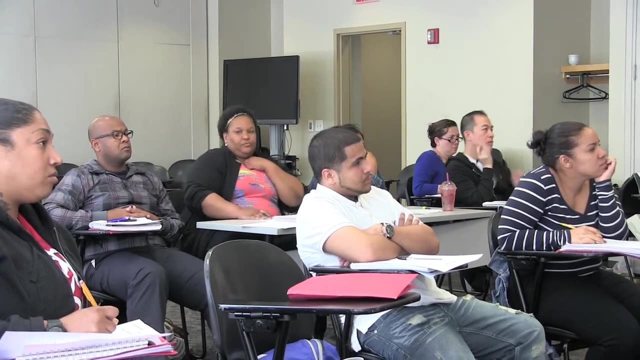 Yep, There's your 13 blocks. Does this pattern? could this be the fourth one? No, No, No, No. I hear, yeah, I hear no. So yes, in the sense that, OK. so one pattern that we saw here: 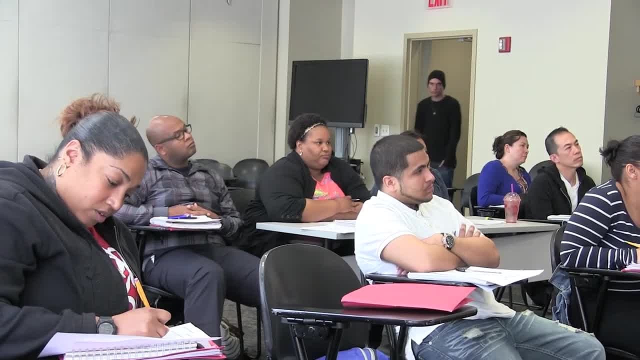 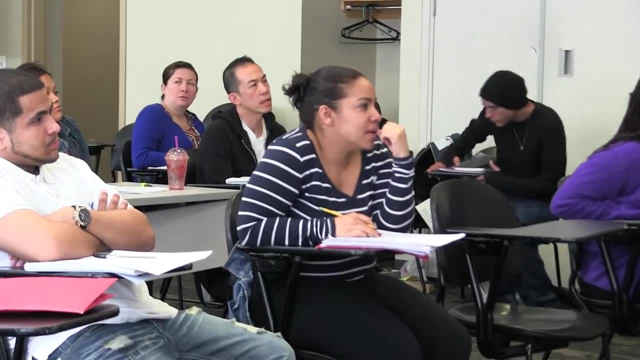 is that the total number of boxes would have 13.. So this is my 13 here. Yeah, but it's not like a form of a T, It's a pattern. It doesn't have to be. It's a pattern, Right. 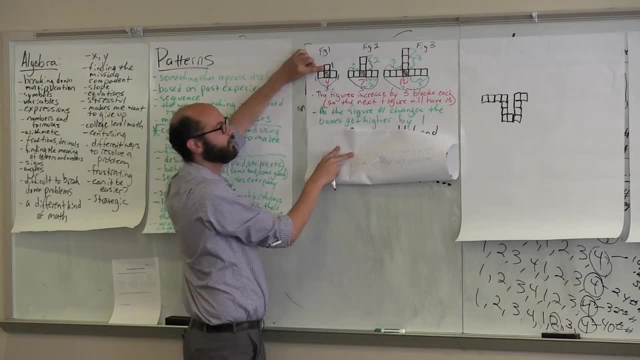 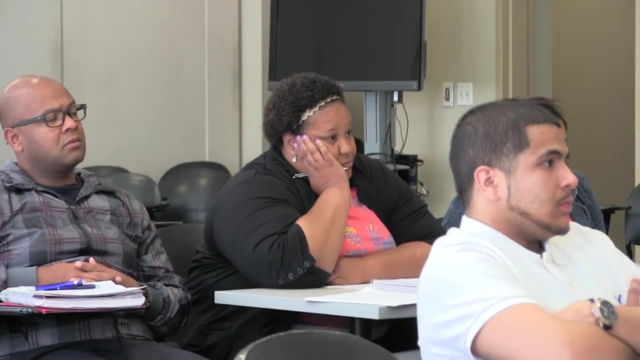 So this is 2, or it's 1 on top, then it's 2 on top, then it's 3 on top. So does this follow that pattern? No, No, There's no. what is on top? This doesn't right. 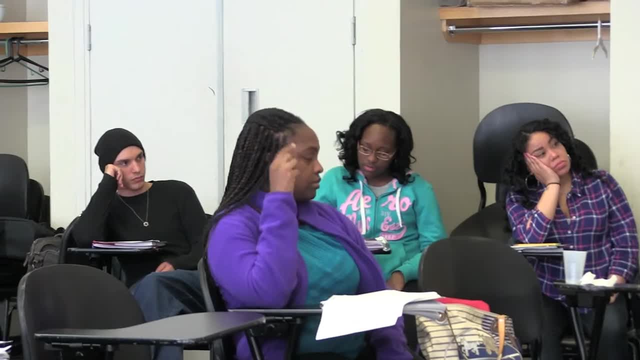 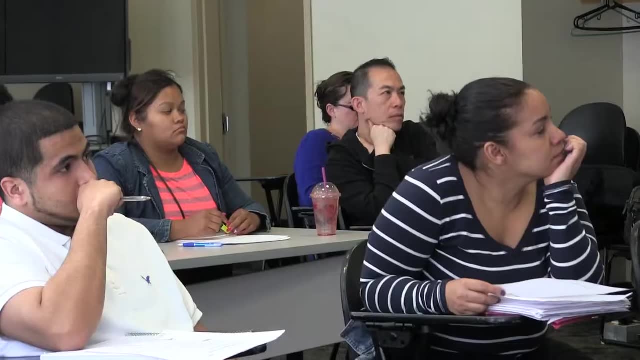 So that's the idea. So all of those things have to be true. So that's why it's important to push. So what are all the different patterns? Because that's your list of things that have to be true when you're making the prediction. 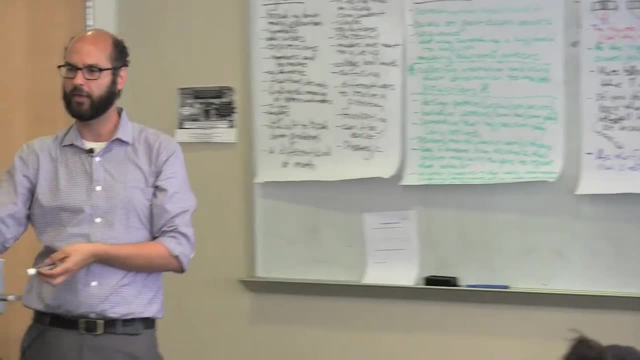 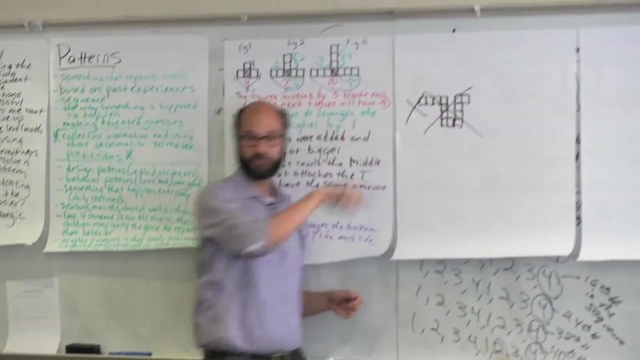 And when you're thinking about, is my prediction a good prediction? Is that the right way? Is that what it looks like? Because we're telling the future right, But in ways that we can say this is not what it looks like. 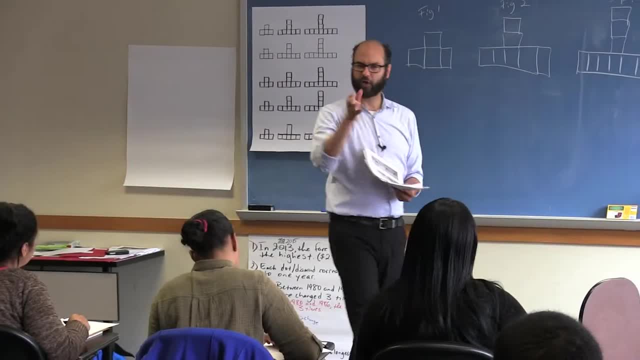 To kind of just remember, there are five different ways that people saw, five different patterns that people had, And so let's see, I don't have enough, but I think you guys can. I think if you're in pairs we'll be good. 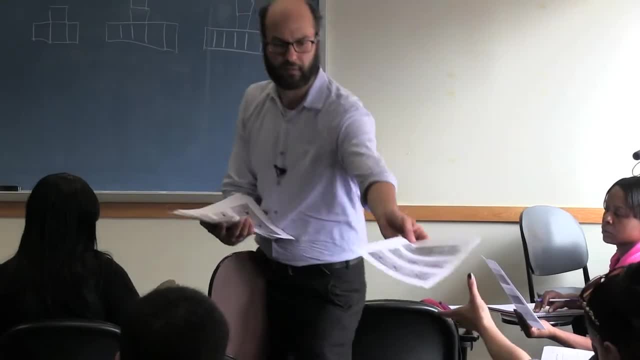 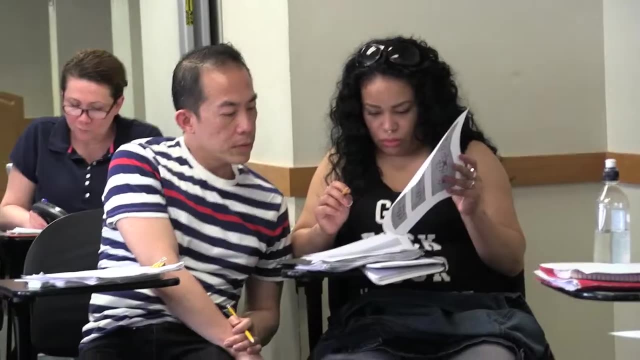 So take a look. When we started working on the upside-down T problem, I had collected all of the different things that they had said, what they saw changing as the figure number changed. So we did an activity where I had them match the written description of their classmates. 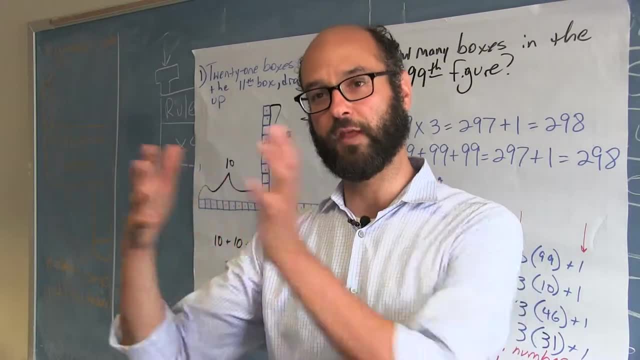 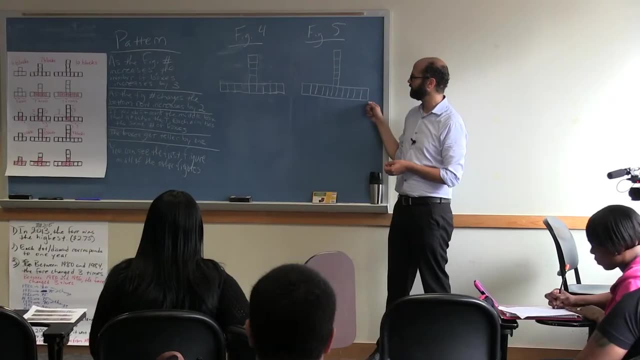 to a visualization. I drew a picture that tried to represent the way each of them was seeing it. It's been a class since we did it, and so I wanted to emerge them somehow back in the patterns. So then we did the next two figures: the fourth figure and the fifth figure. 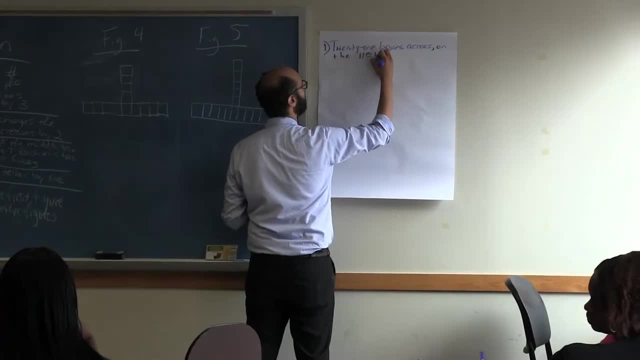 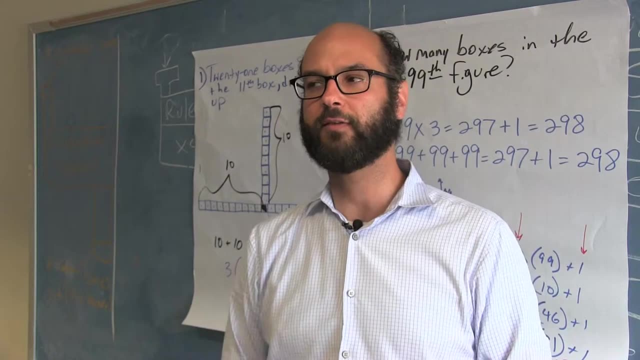 And then it's the tenth figure, and that's kind of where a lot of stuff starts to happen, because once you get to the tenth, you could draw it, but you're, you know, we're at the edge of kind of where we want to start thinking of other ways. 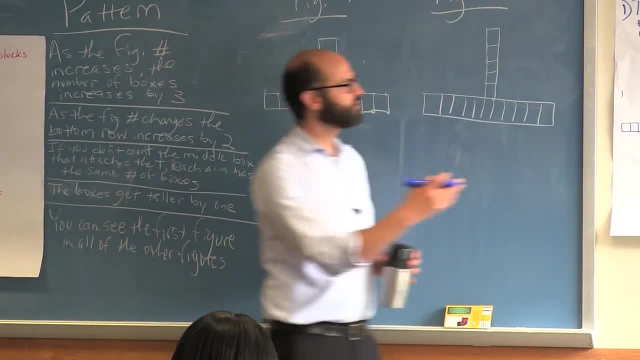 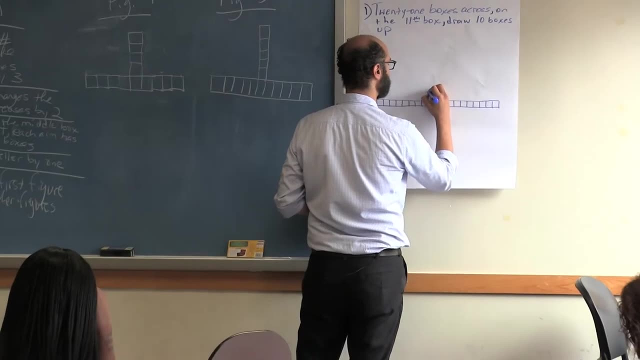 Twenty-one boxes across. Now she said to go to the eleventh box: One, two, three, four, five, six, seven, eight, nine, ten, eleven, And then draw ten boxes up: Two, three, four, five, six, seven, eight, nine, ten. 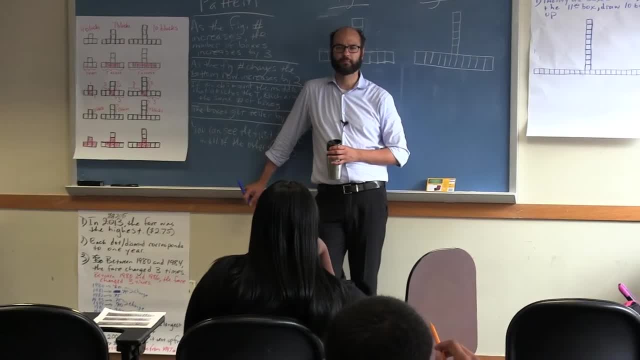 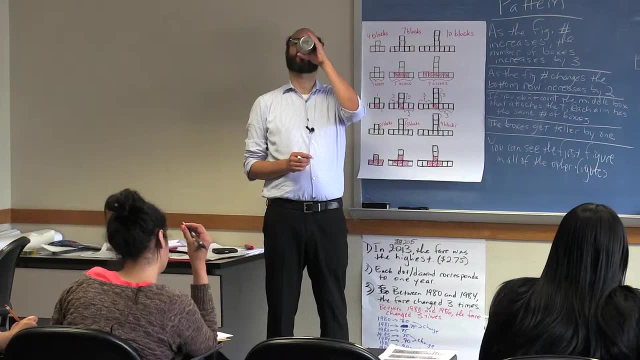 That's the picture she said to draw. That's what I got, Is it right? Is it right? I don't see it. Anybody have any Any ideas? Add three, five more times. Add three, five more times. 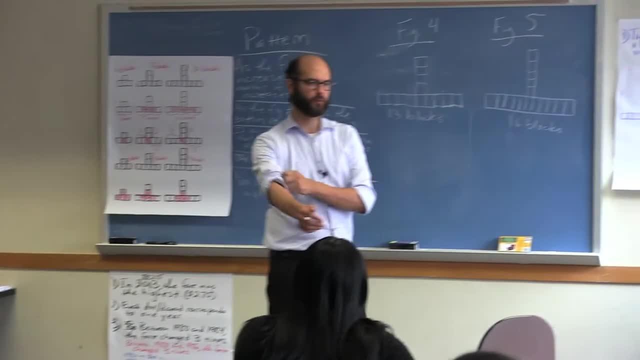 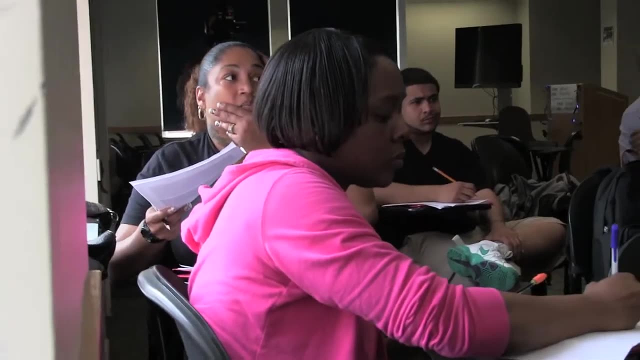 Talk to me about what you mean by that. Figure six will be nineteen. Ah, so we can build up. Yes, Okay. So one way that, if we're going to do that, one way that's useful, a tool that's useful for doing that is to kind of- is to set it up in a chart. 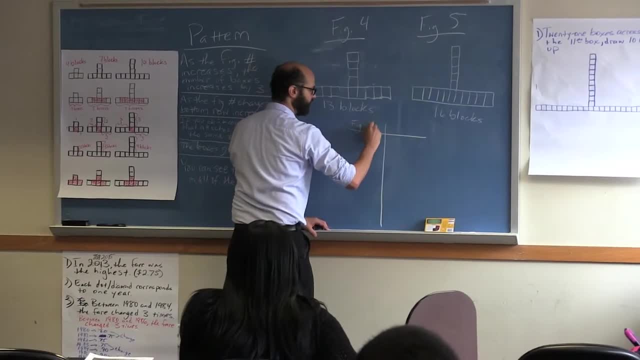 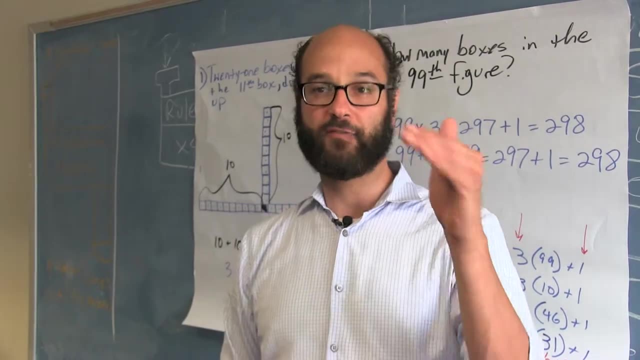 What I wanted to do was a couple of things, and they both happened. One: I wanted to get the idea of a chart- Roxanne focused on that one- where each figure has three more blocks than the one before, And we had five, so we could figure out the ten by just saying the sixth would have three more. 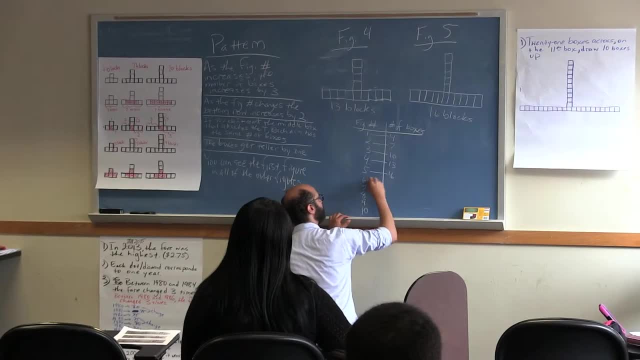 and the seventh, would have three more all the way down to the tenth, And so that's a good strategy that I wanted up How many would be in the sixth figure: Nineteen, Nineteen in the seventh figure: Twenty-two. 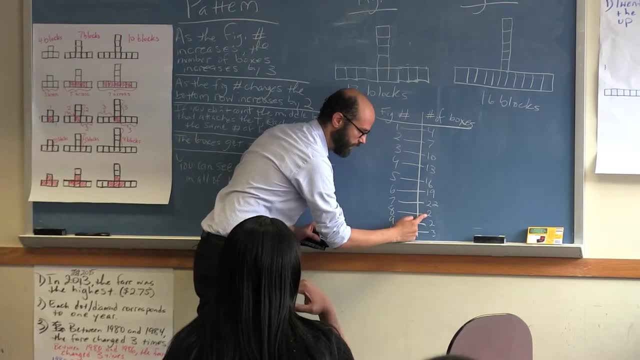 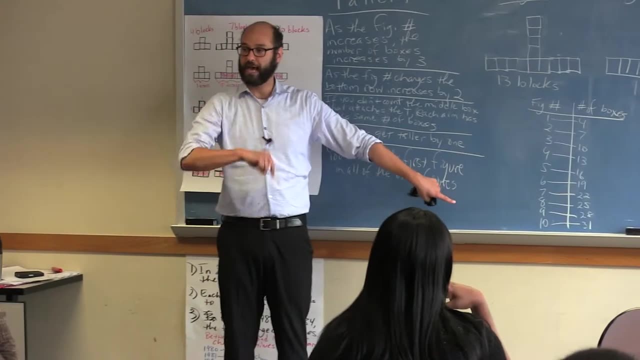 Twenty-two, So twenty-two, then twenty-five, twenty-five, twenty-eight, Thirty-one, Thirty-one, So the tenth one should have thirty-one. Did we use any of the other patterns that people said, The ones that people saw, to help us with this one? 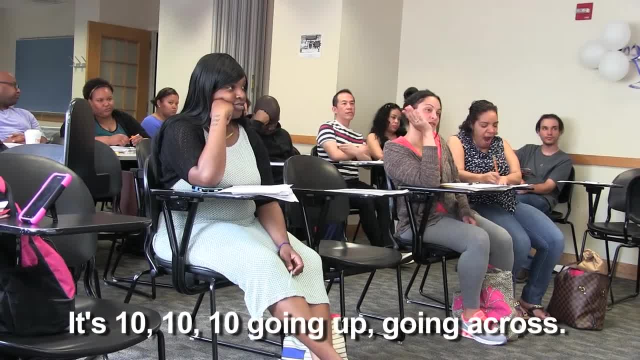 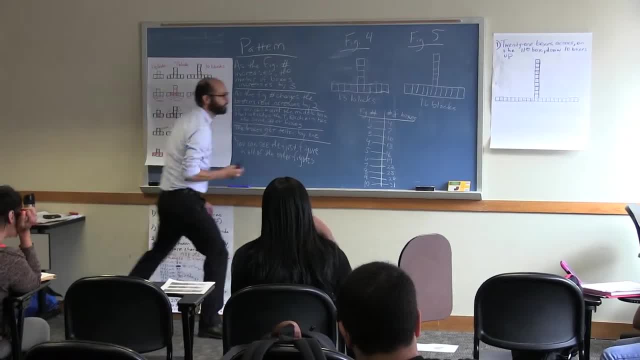 No, everything was even with ten, ten, ten one up, one one. So okay. so I mean back it up and say that. But I also wanted to lead this towards generalization. Sabrina had me draw twenty-one and then on the eleventh, go up ten. 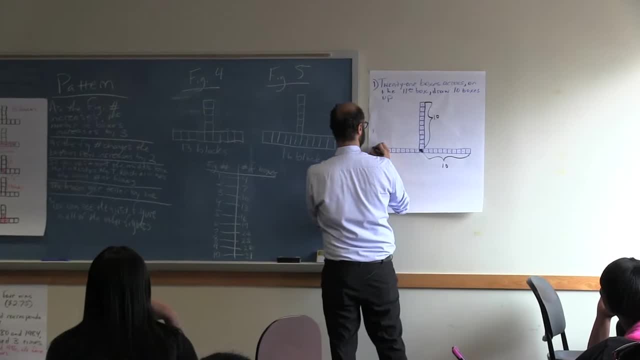 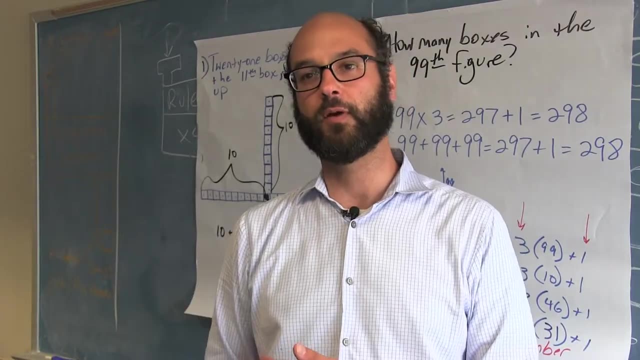 And what it ended up being was a picture. If you ignore the one in the middle, you've got ten, ten and ten, And that was going to lead them to the generalization that we eventually got to, which is three times the figure number plus one. 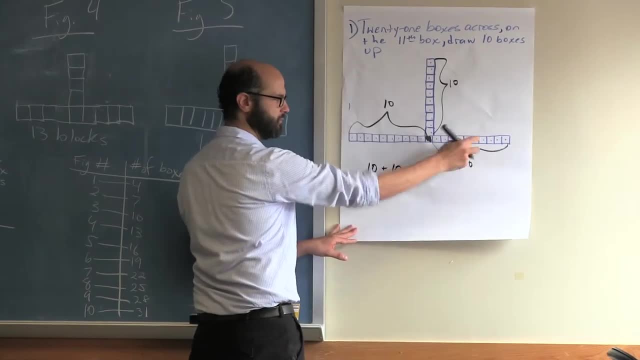 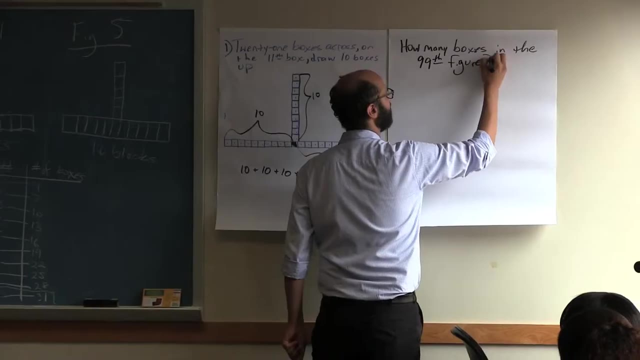 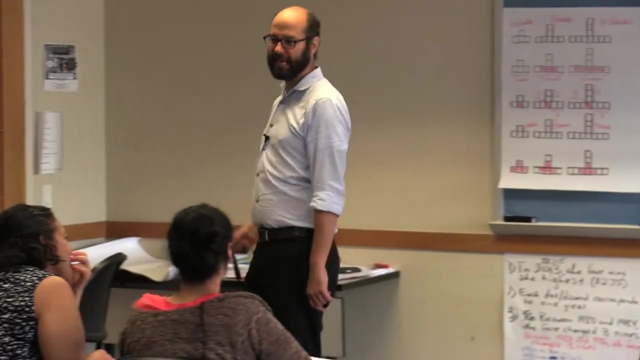 Ten plus ten Plus ten Is thirty Is thirty plus that one in the middle Right Is thirty-one. Okay, So I want to know how many boxes would there be in the ninety-ninth figure? Ninety-ninth figure. 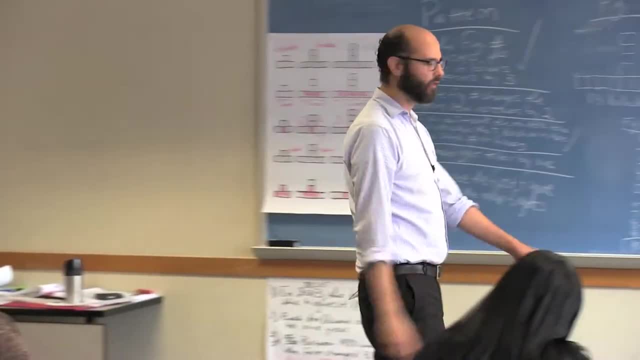 Take a minute, don't call it out, just take a minute to think about it. So I asked them the ninety-ninth and I kind of gave them a couple minutes to just kind of use the picture that we had of the tenth. 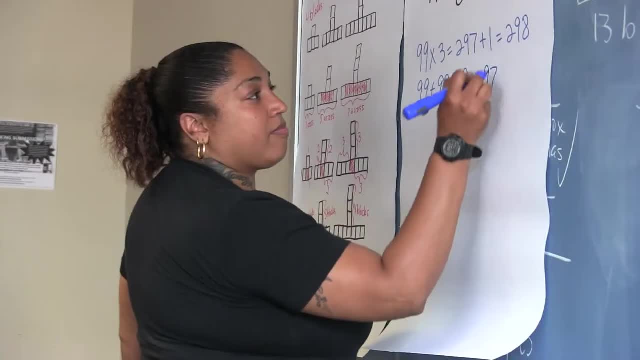 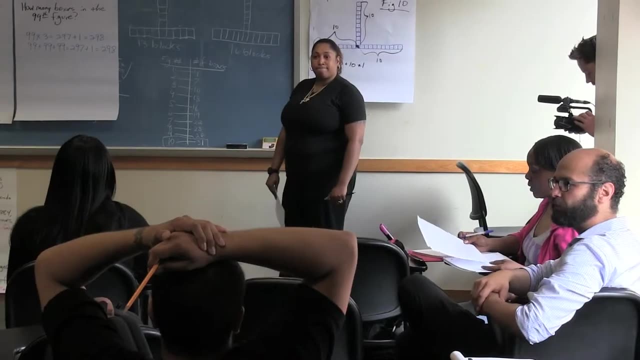 And then I had one of the students come up and show her strategy, and it was great because she wrote both Three times ninety-nine plus one and ninety-nine plus ninety-nine plus ninety-nine plus one, And so we talked about where each of those numbers came from and why it was three of them. 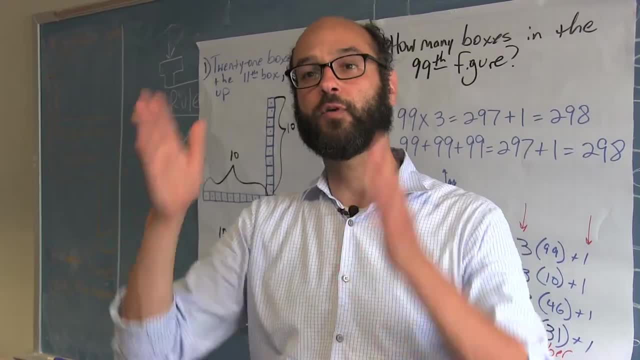 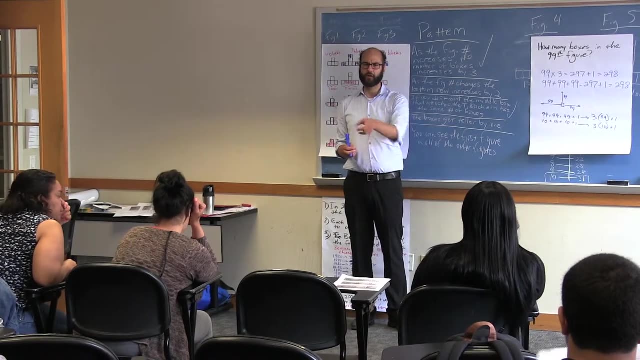 And then I said: okay, so what would you do for the forty-sixth, For a series of numbers and I had them all written. So how about the forty-sixth figure? The forty-sixth is one thirty-nine. How did you figure it out? 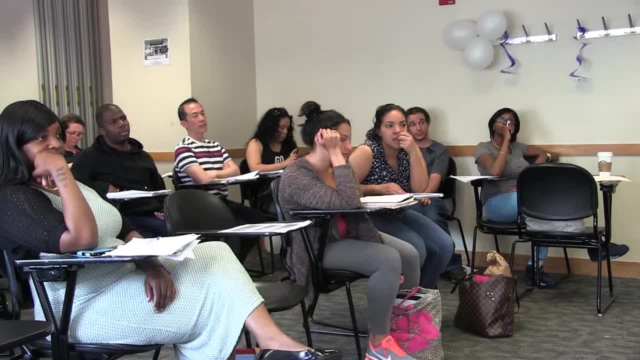 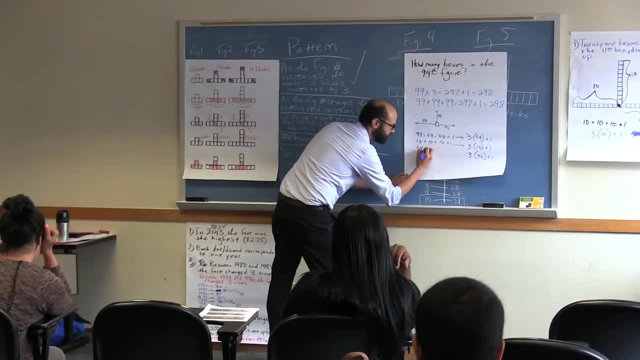 Three plus one. So what do you mean by that? So three times the forty-sixth plus one, or how can we write it this way: Forty-six plus forty-six, Forty-six plus forty-six, Forty-six plus forty-six plus forty-six plus one. 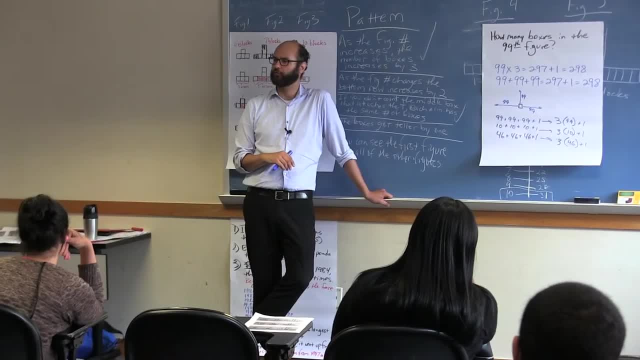 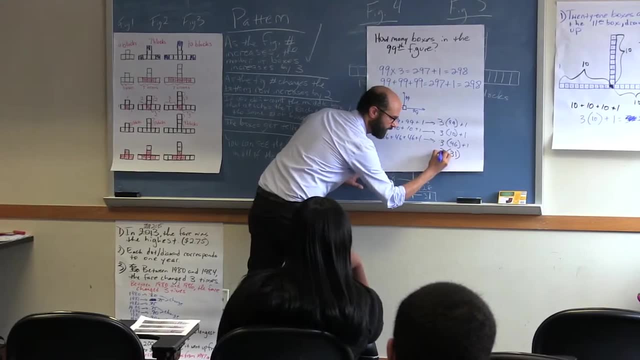 So if we want to do the thirty-first figure, if I wanted to know how many squares are in the thirty-first figure, how would you do it? Thirty-one times three, Thirty-one, the figure number times three Plus one. As you look at these, what's changing and what's staying the same? 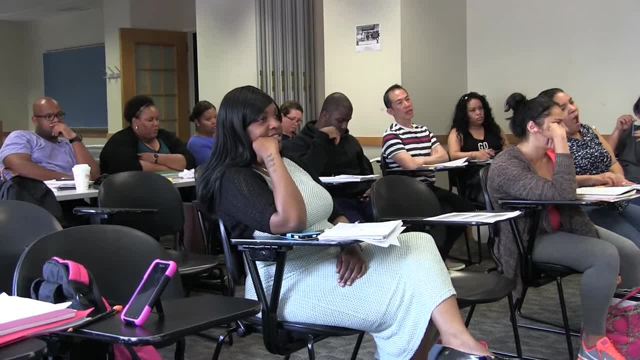 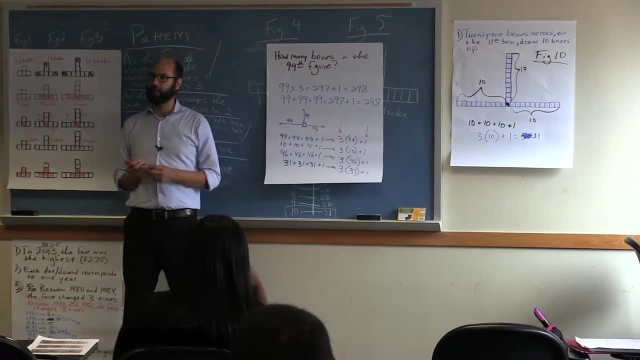 The three stays the same. So the three and the plus one. So the three and the plus one. So the three and the plus one stay the same. and then what's changing? The figure number, The figure number, The figure number. 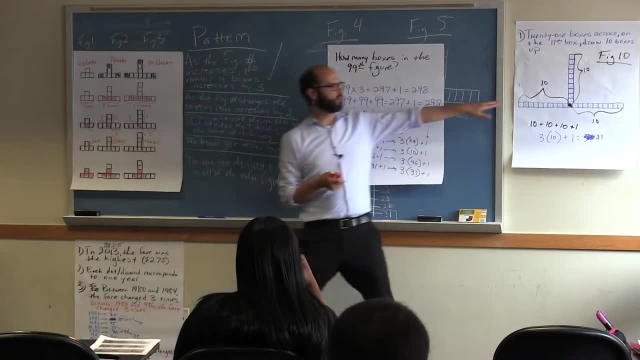 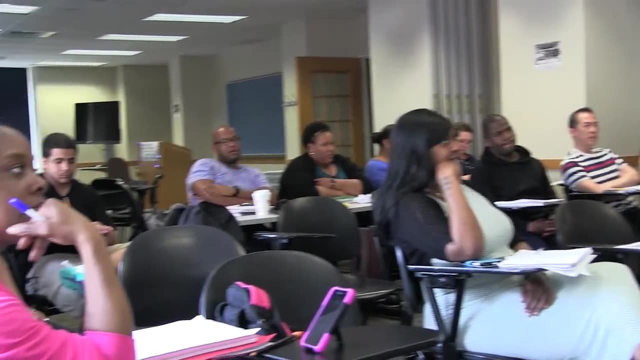 This is the figure number right. We asked for the ninety-ninth figure, for the tenth figure, for the forty-sixth figure. So, whatever number I give you, what are you going to tell me? Times it by three. Times it by three. 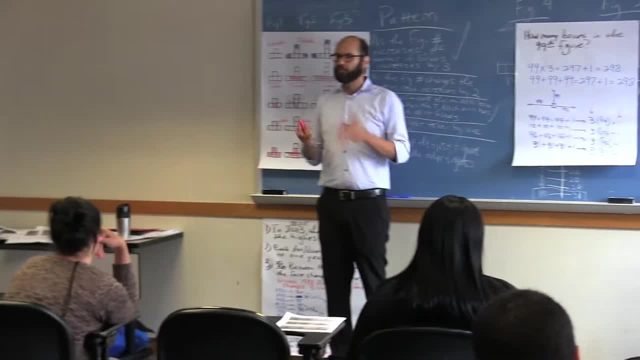 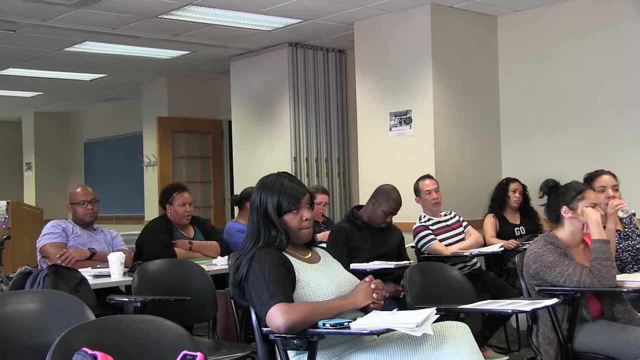 Plus one, Plus one, And then add one, So for any number, Yep. So does anybody know a way that you can? how do I write it? I could write this. I could say: multiply the figure number One, One. 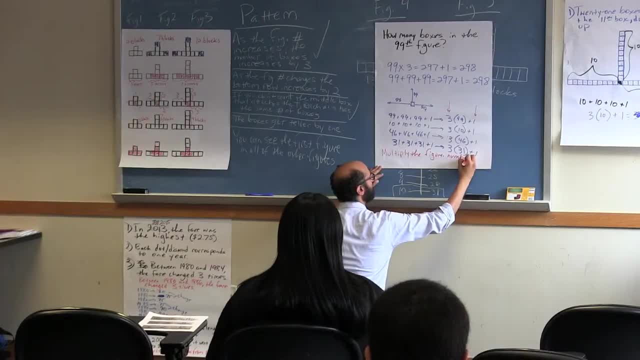 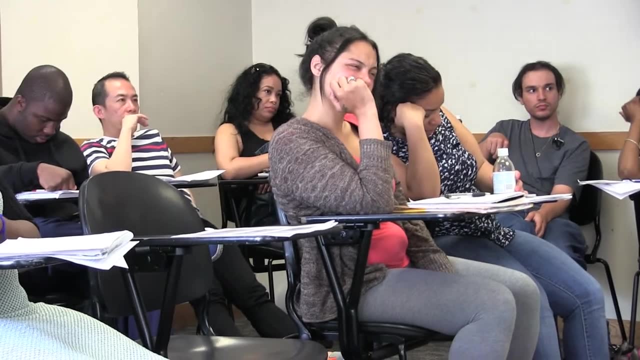 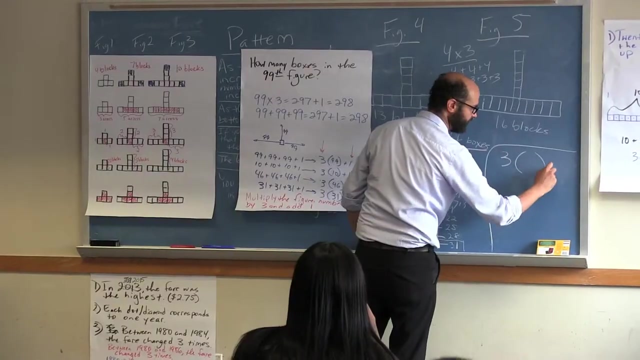 The figure number by three and add one. Is there a short way to write this, A math way to write this, A scary way to write that? It's going to be three times something plus one, right, This is the part that's changing. 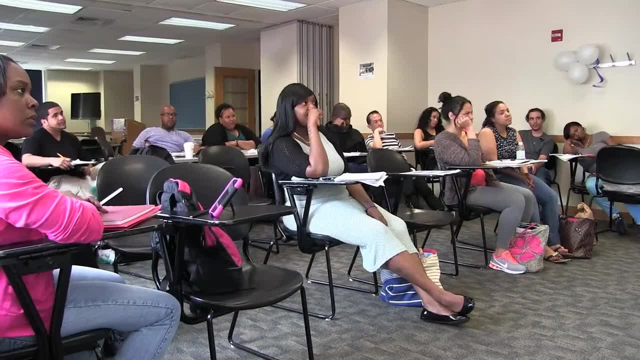 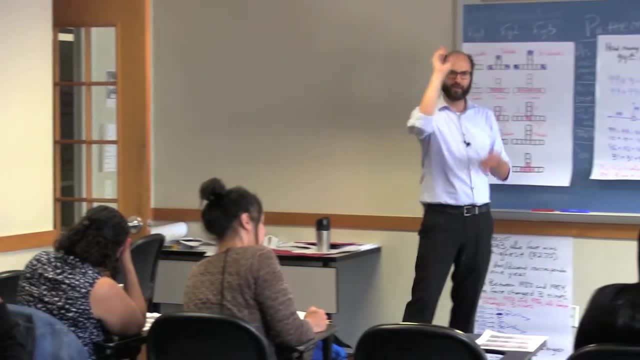 What's another word for change? Change Variance, Variation, Variant Right. When something changes, it varies. It changes from one to the other. Does that ring any bells? Does that sound like any math word? maybe you've heard? 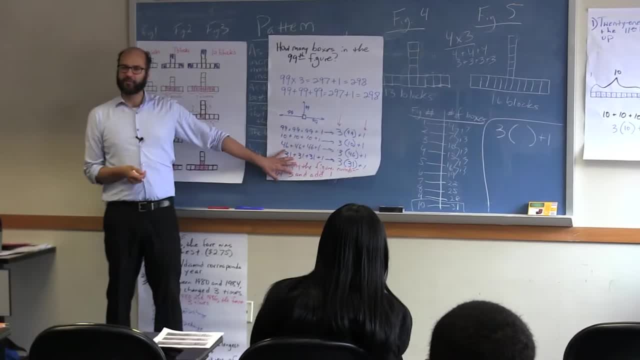 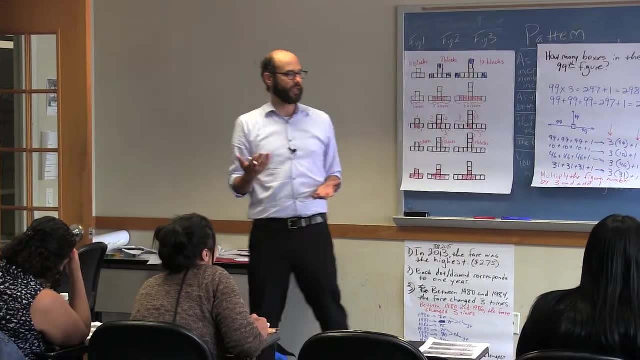 Variable, It's a variable. One way to write this is I can say: well, take the figure number and any figure number you get, multiply it by three and add one. Right, But that's a lot to say and certainly a lot to write. 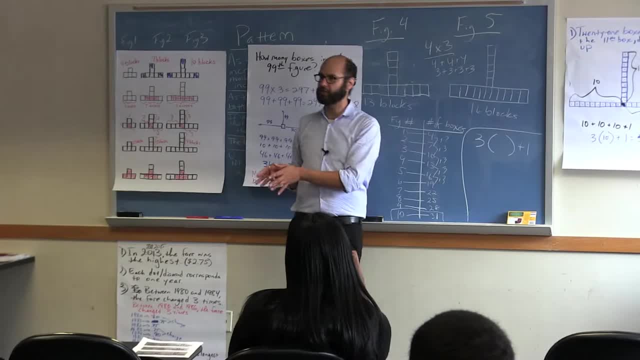 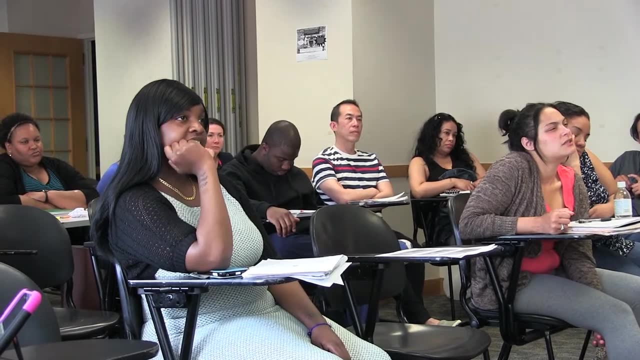 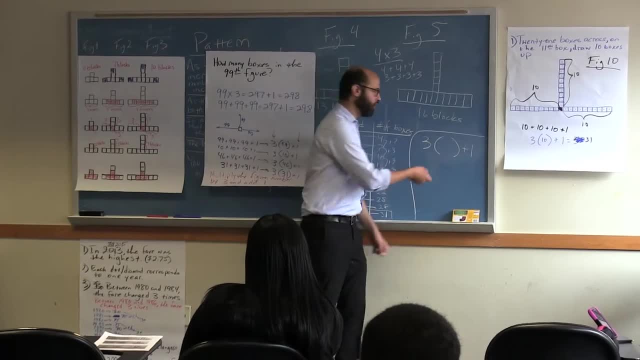 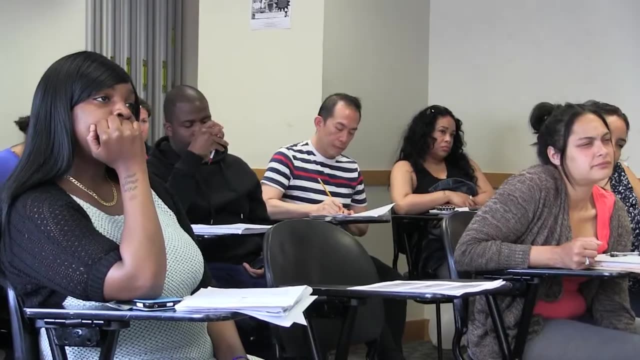 Times it by three, or add it to itself. three times M plus one, Add it to one, right? And this is what we're going to do with it, right? So, rather than saying any number, we can just pick, let's pick m. 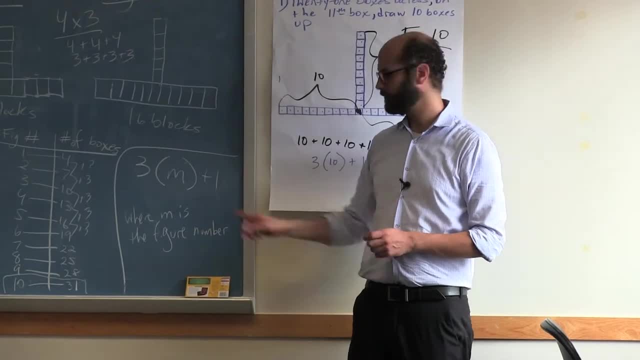 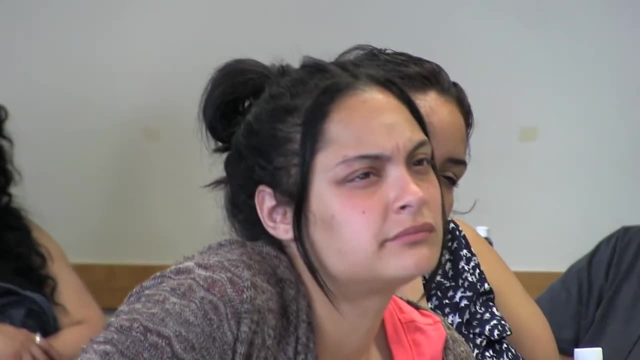 Where m is the figure number. So, whatever the figure number is, you're going to multiply it by three and you're going to add one. I know adult education students struggle with in terms of algebra is there's lots of different uses of variables. 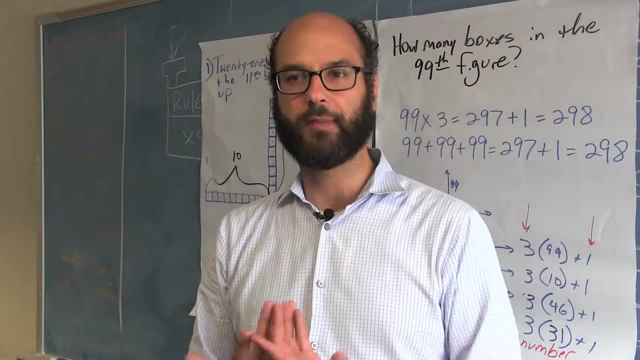 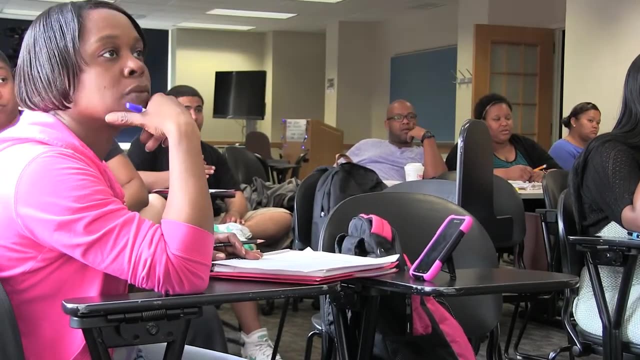 but I also wanted to lead this towards generalization. I wanted to root it in this visual so that it could be rooted in something that's concrete, because, eventually, what I want is for them to keep internalizing that question of what's changing and what's staying the same. 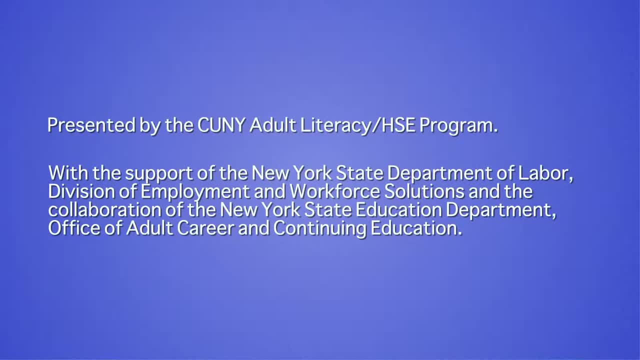 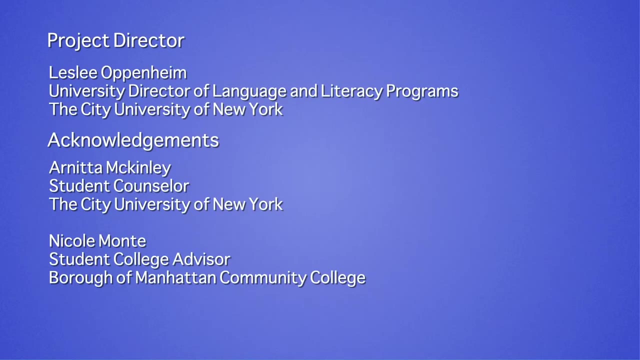 When they look at the next picture. I want them to have that question. Subtitles by the Amaraorg community.